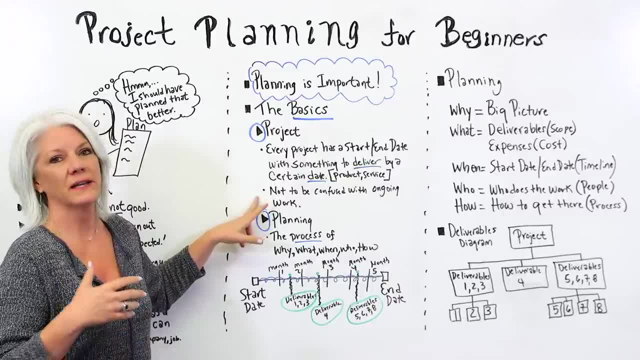 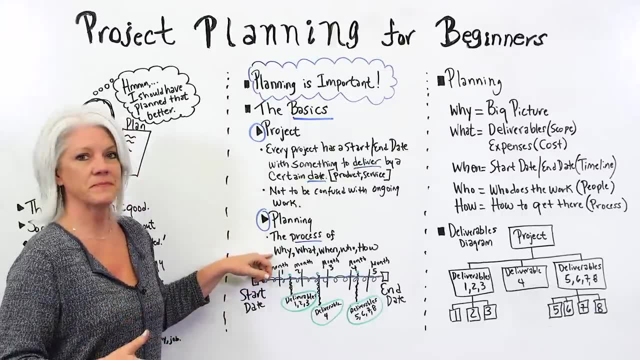 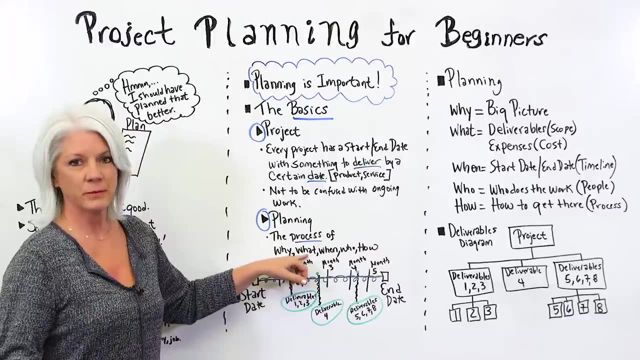 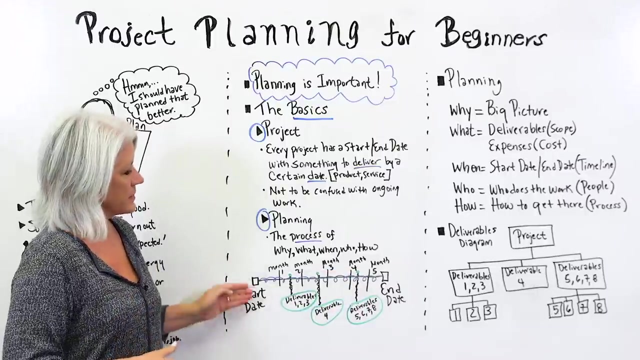 So it's not to be confused with ongoing operational work. So in planning, planning is a process of delivering. you know why are we doing this project ultimately, What's the ultimate deliverable? What other deliverables are going to be produced, like what product or service? Who's going to be involved in doing it and how are we going to do it? So, if we look at a graphical picture, we've got a start date and we've got an end date. 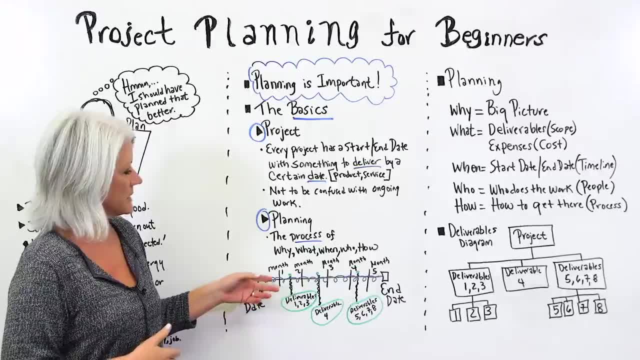 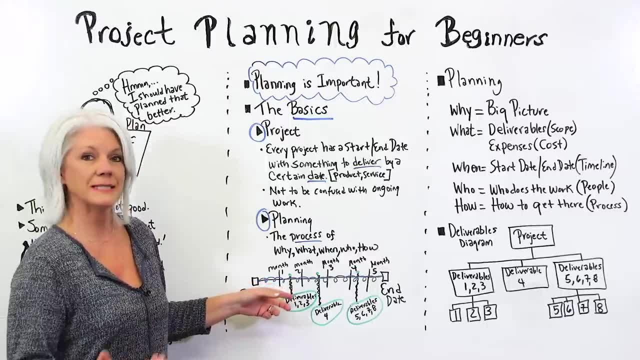 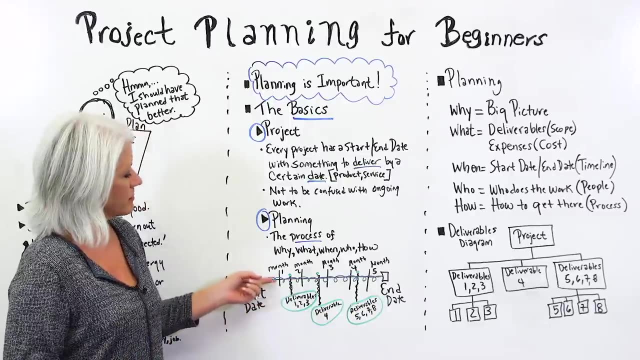 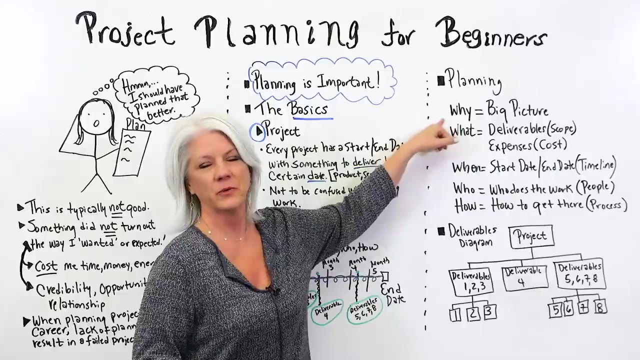 Maybe we have different chunks of time. This specific one is by months. We've got five months highlighted And then we have different deliverables according to different points in time. We could have three deliverables due here, one delivered here and maybe four here, And then there's the process of how we go about doing that. So let's look at planning. So planning again- we're talking about why are we doing this project? What is the big picture? 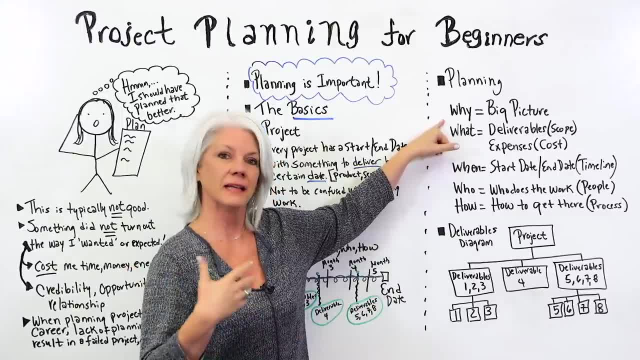 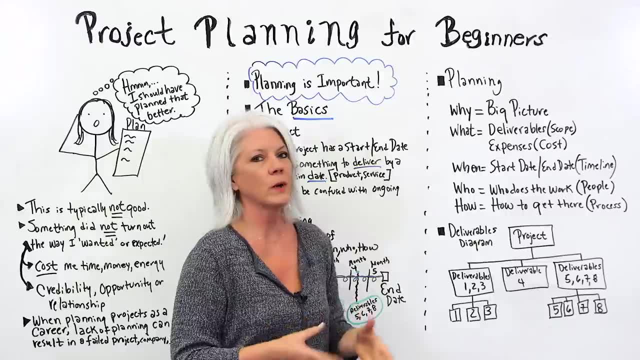 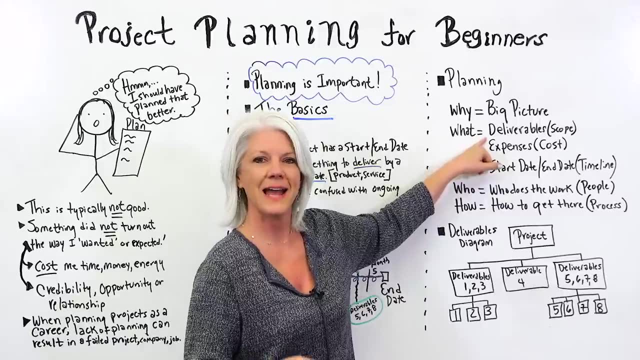 What are we delivering from a high level? Is it like a building? Are you delivering or planning a wedding, Something like that? And then, what specific are we delivering according to deliverables, And in some places you may hear that referred to as scope. 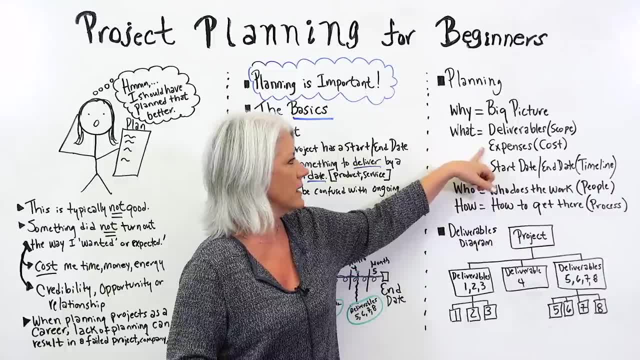 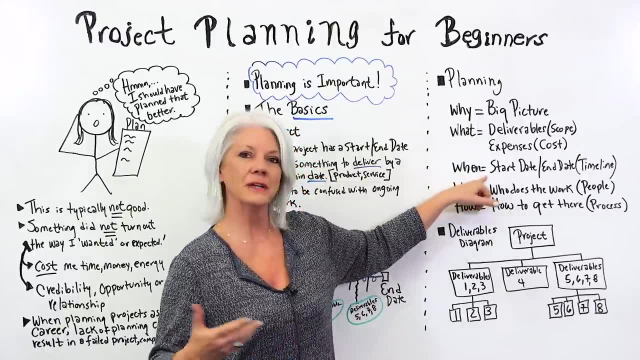 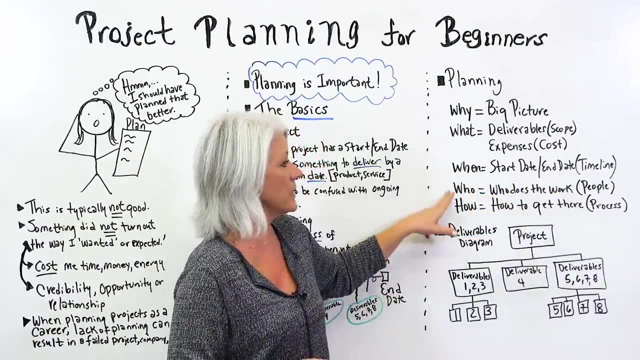 We also, as a result of the project, will have the expenses, And those are compiled to our project cost. Then we look at when- okay, When is the start date, When is the end date, And that creates our timeline. We also look at who actually does the work. 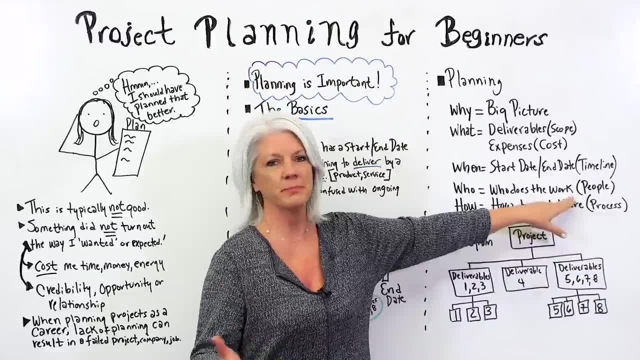 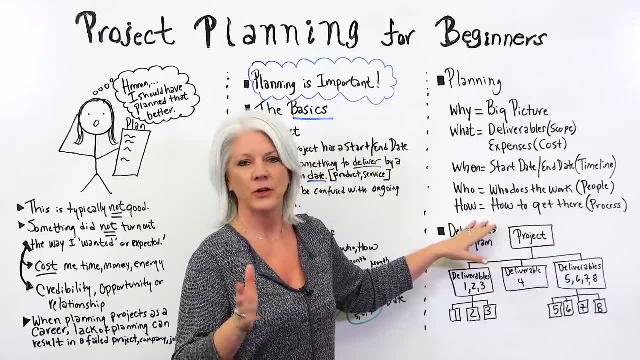 to deliver the products or the service. So those are our people resources. And then, how do we get there? What is the process? How do we know on the project, Who knows what to do, when and where? There's got to be a process. 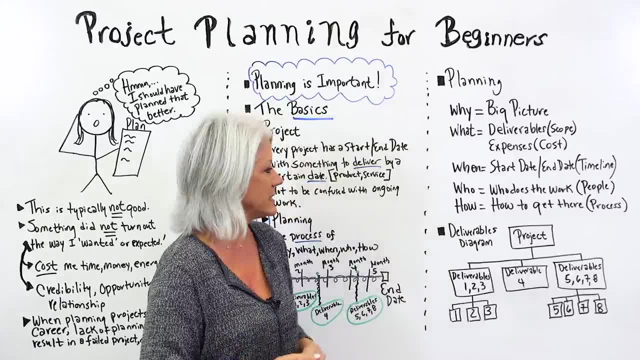 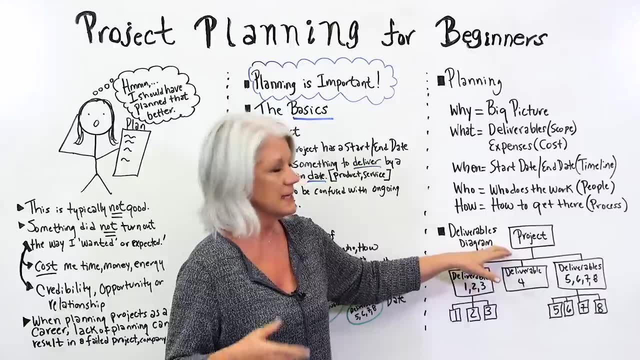 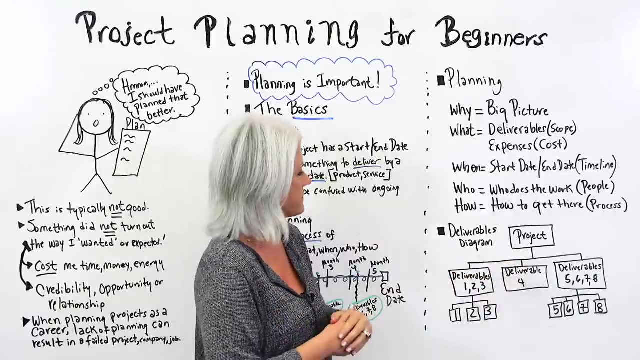 So one of the most valuable things I've found in planning is what's called a deliverable. A deliverable is a big picture of what we're ultimately delivering. Again, I love using the example of a house. So ultimately the project may be, you're building a house.